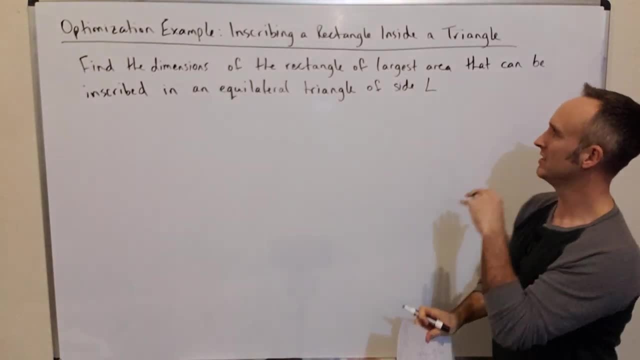 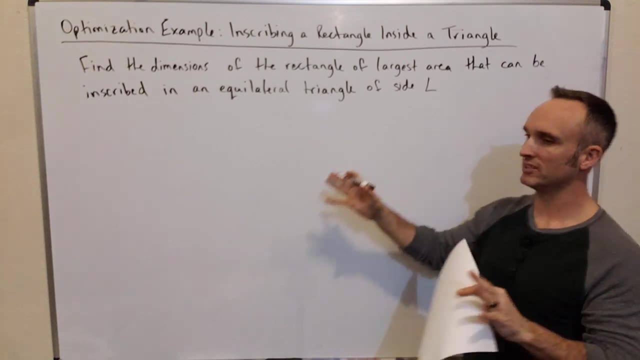 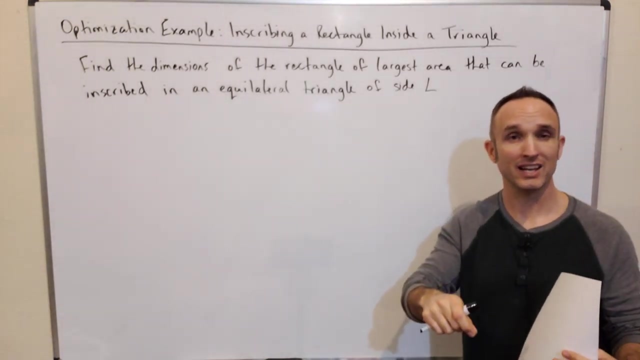 capital X. One thing to keep in mind here is that L is acting as a constant in this problem, And the idea is, anything we solve for this will have L in the answer, so that if we wanted to change the size of the triangle to a different L value and plug something specific in, we 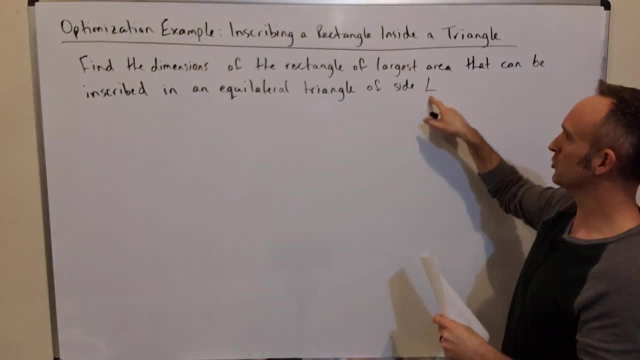 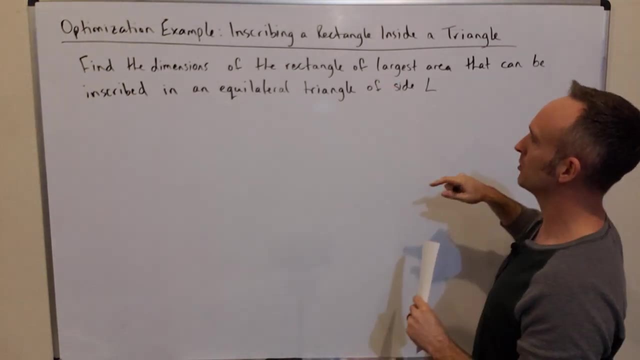 could modify our answer for that particular L value. So we're going to treat this as a constant throughout the duration of this problem. So we're inscribing a rectangle in an equilateral triangle of side length. So we're inscribing a rectangle in an equilateral triangle of. 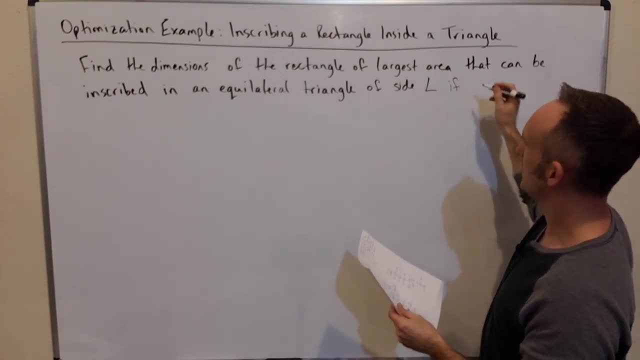 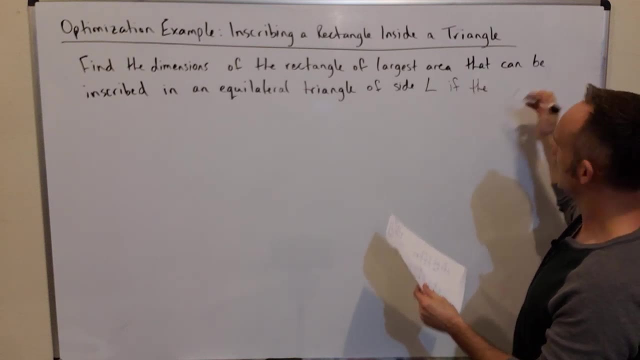 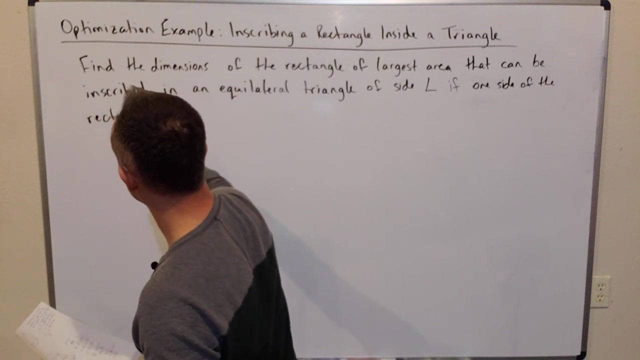 side length L, and we want to, let's see, maximize the area of the rectangle if one side of the rectangle lies on the base of a rectangle, and we want to maximize the area of a rectangle if that rectangle is not on the base of that rectangle. And if we want to maximize the area of a rectangle, 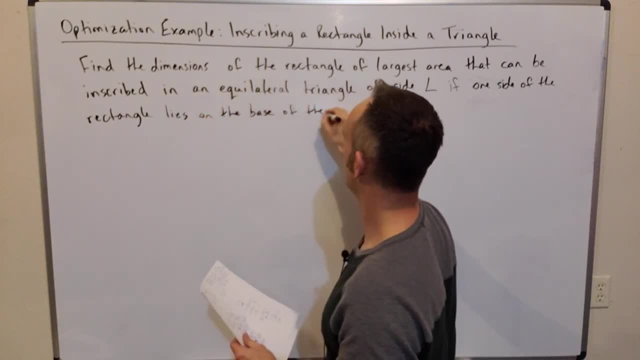 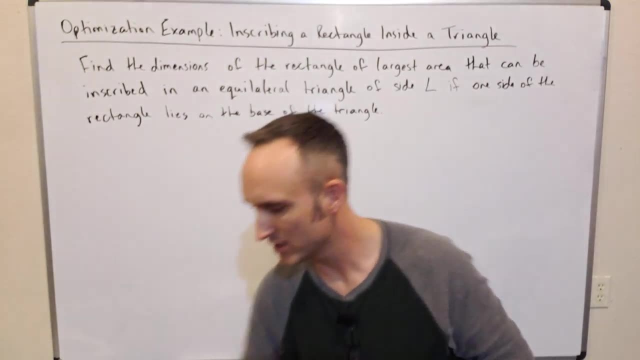 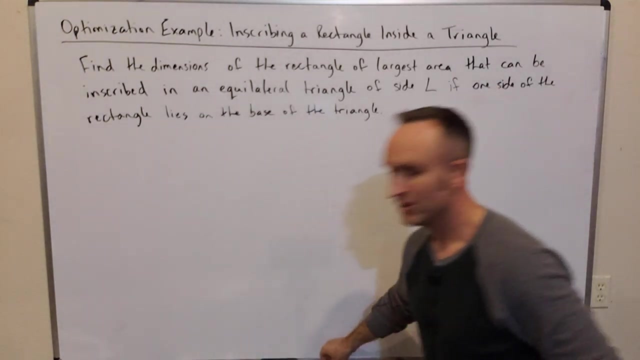 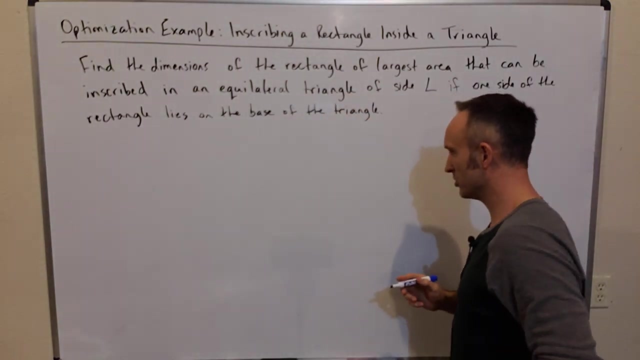 of the triangle. okay, so we need to put a rectangle inside the triangle, so that one side of the rectangle lies on the base of the triangle. okay, a lot of words there. let's see if we can describe what's going on with a picture, and I will. I will draw this picture over here this time it's got. 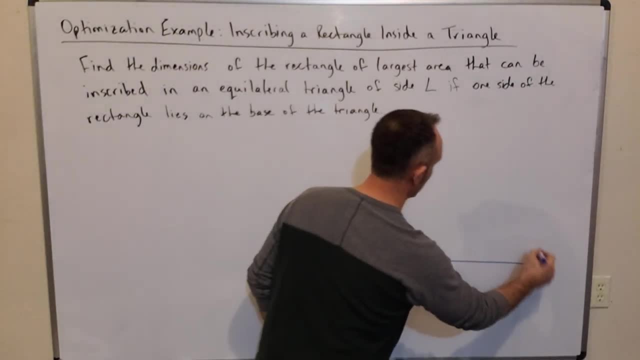 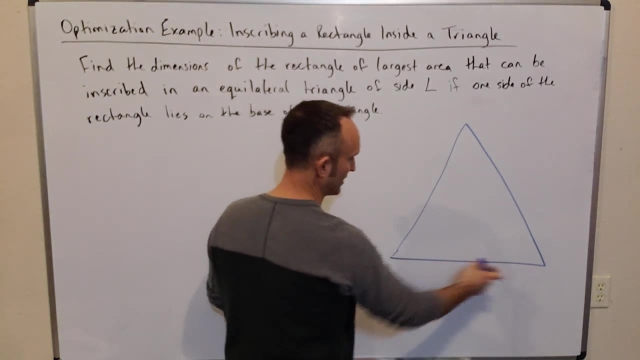 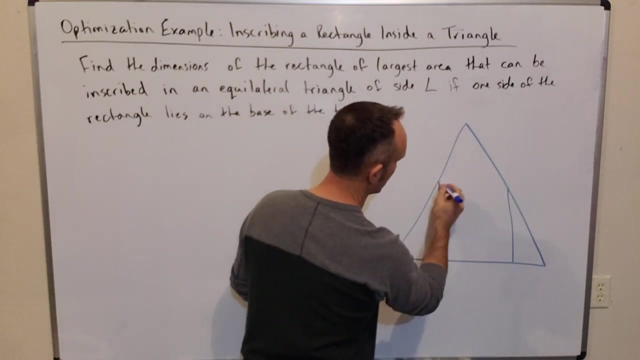 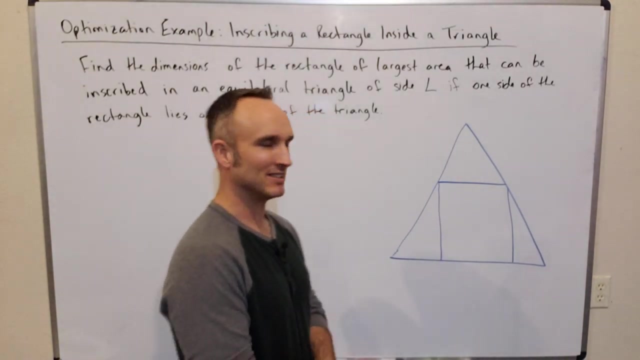 to be pretty large. so I've got my equilateral triangle here and my rectangles inscribed inside, and one side of my rectangle lies on the base, so any rectangle I draw might look something like this: let's, let's pretend that's a rectangle, right? so this is our rectangle. we want to maximize the. 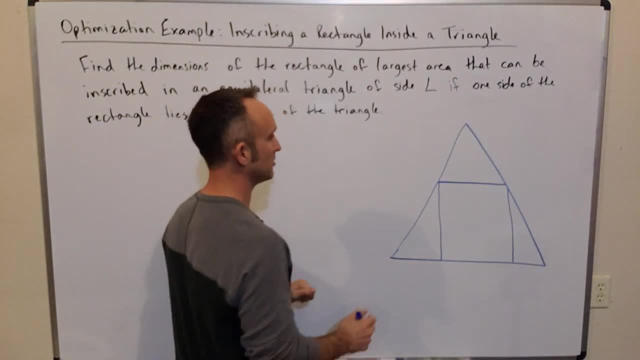 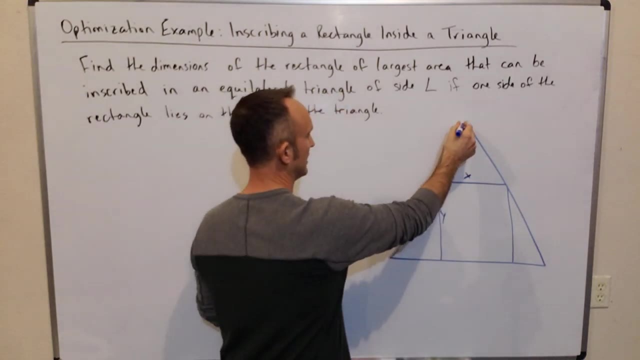 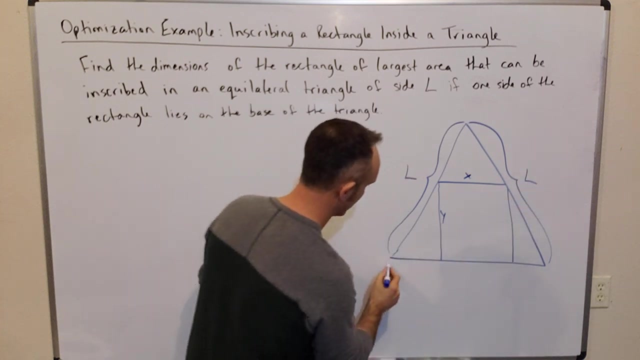 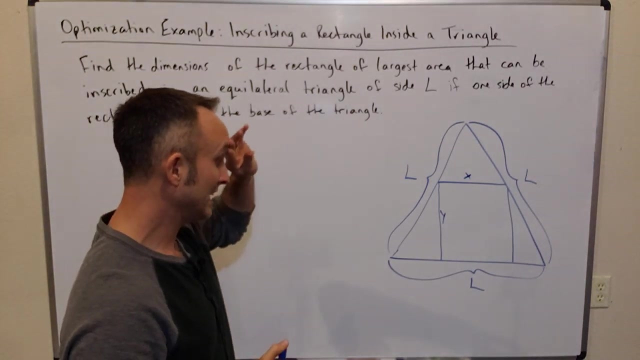 area of that, and we're asked for the dimensions of the rectangle. so maybe let's go ahead and call this length X. in this length Y, let's indicate that the lengths of the sides of the triangle are all L, and that's what we're given, okay. so what I need is some. I need two things I need to know. 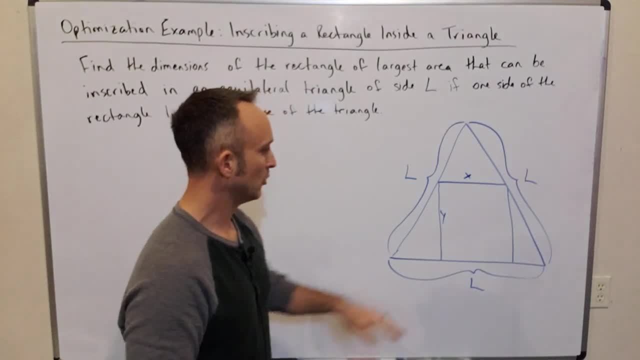 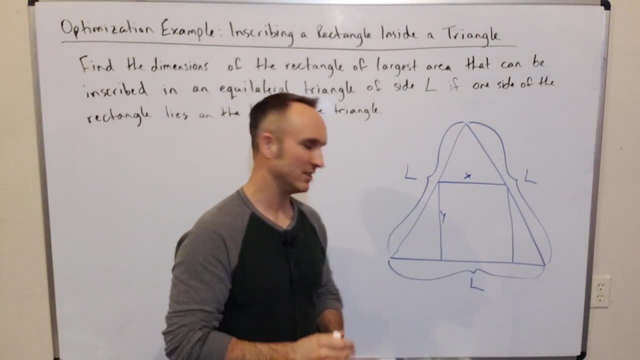 the relationship between X and Y, if I can. it will possibly involve L, because L is the constant here, like maybe L was 10, right, don't think of it as a variable, think of it as a constant. but X and Y here can change, while L stays constant because the dimensions of this rectangle 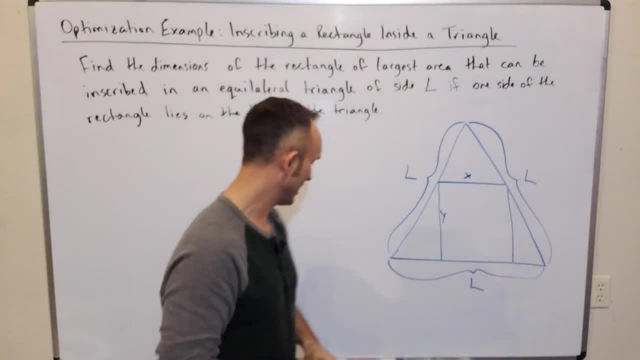 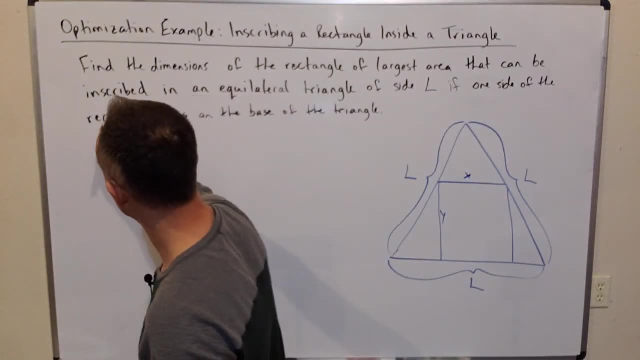 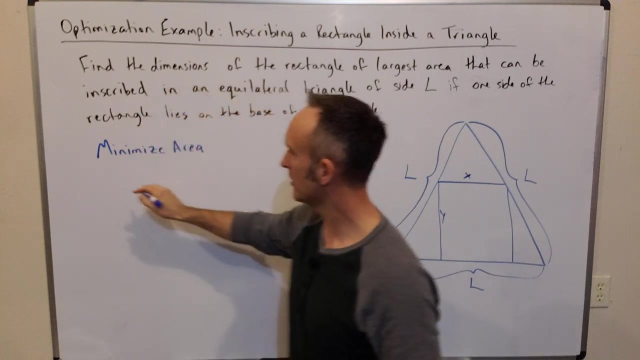 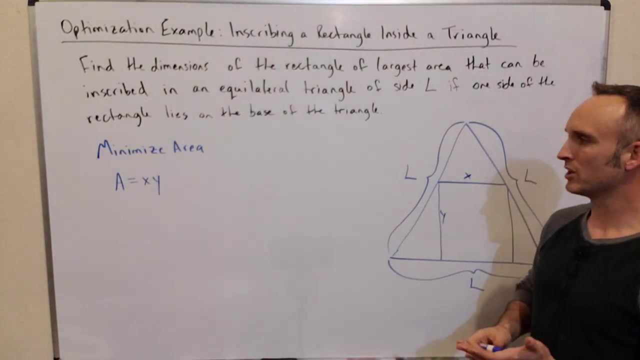 can change and we're trying to find the dimensions that yield the maximum area. so if we're looking to solve this, we know that we're looking to minimize, minimize area and we can describe the area of that rectangle very simply as X times Y. so no problem there. the issue comes when we try to write this: 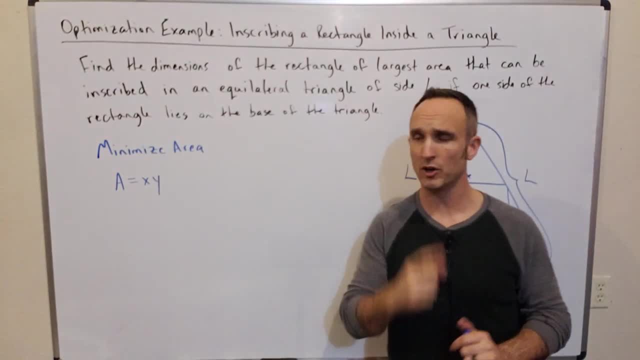 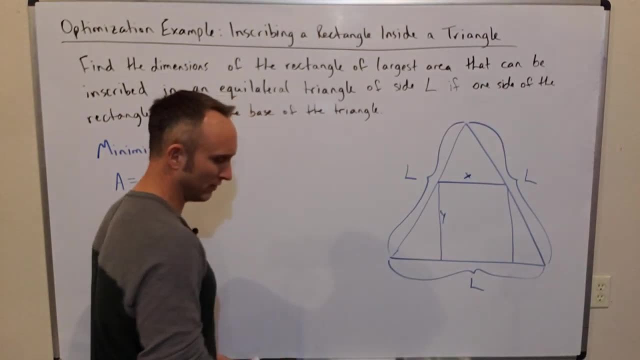 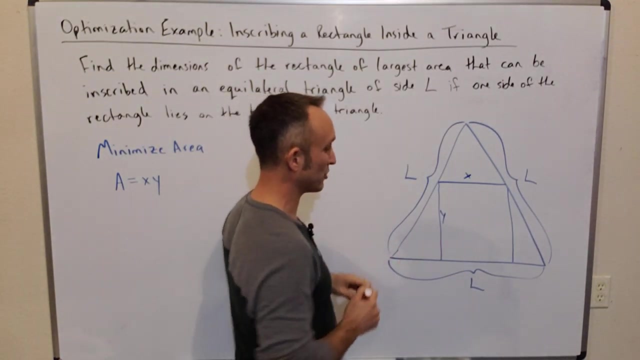 function this area function in terms of X or Y, one variable only, and that's where we have to do a bit of work over here. so let's, let's sort of develop an understanding here. how do X and Y relate? I mean, they're just sides of a rectangle. well, they also fit inside this triangle. so one thing we might. 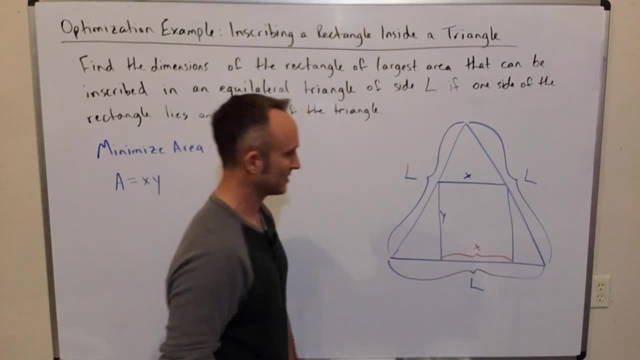 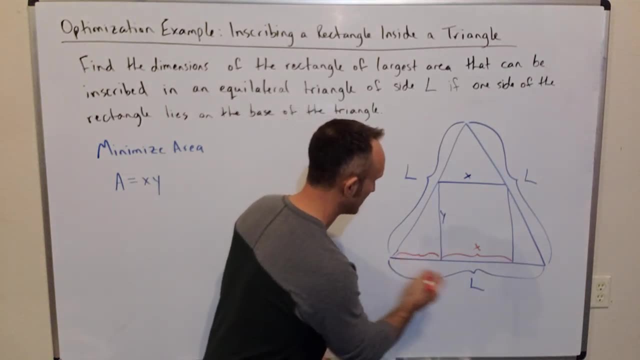 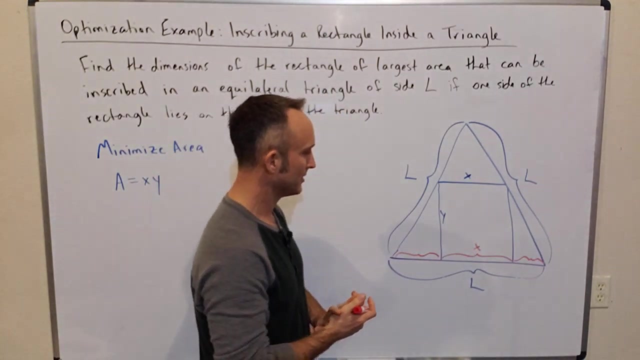 also consider to do one by taking oureles, and we know they're just sides over here, so of course we're gonna multiply those by a者, by the power of the Strang Video. alright, so now, if I can do one size plus one minus one in terms of Y plus one, Y times Y, so this is actually easier than I think it is. 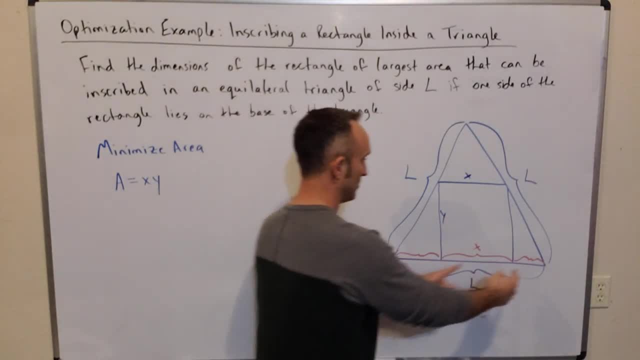 and then if we can find the biggest difference that we can over here- as you can see, over here you read this tower is 21 plus Augustmark times. we know how to write a total length, pessoa plus Y, and we can do one і plus y in order to write the answer hill. okay. so since we've weighed the whole along, we can. 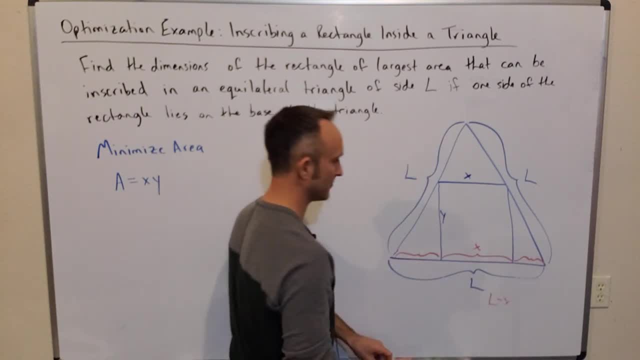 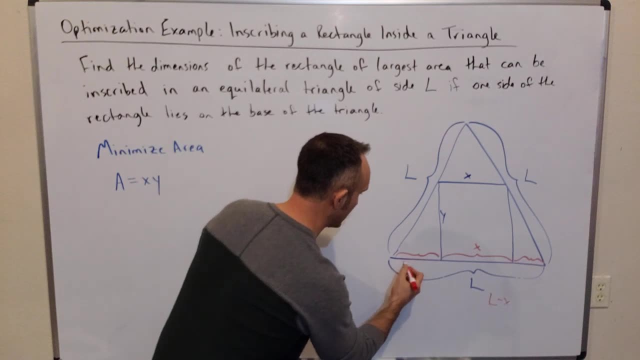 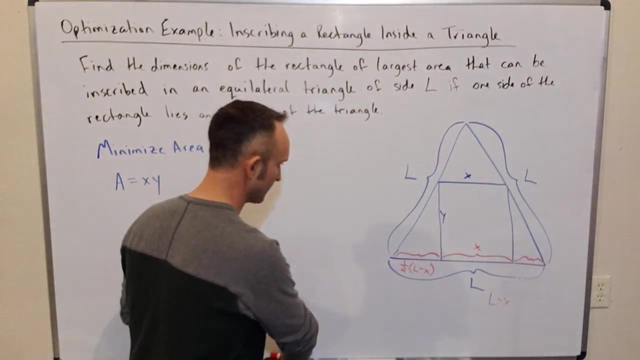 two guys have to add up to L minus X, right? Because if I take L minus this piece, it leaves behind those two. So in other words, I know that this length right here is one half of L minus X, and so is this over here. Now I'm going to focus on one side, because both of these triangles are 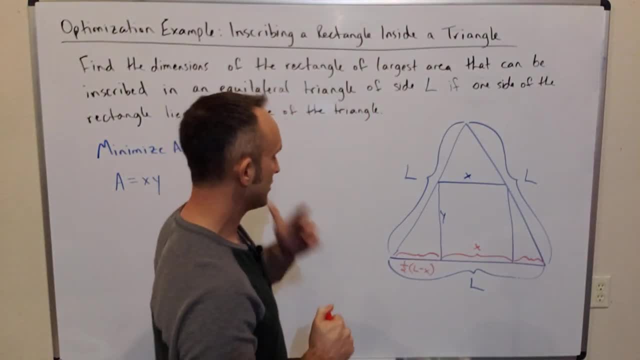 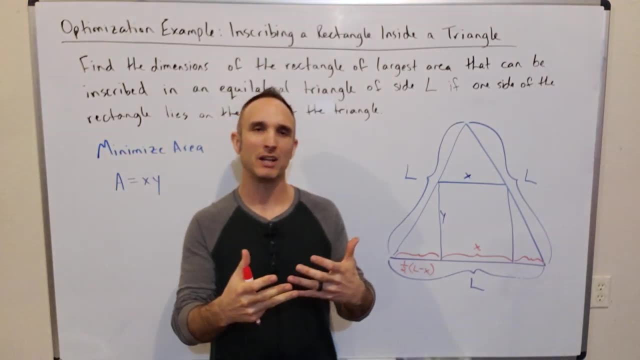 exactly the same. They're congruent triangles. Now, once I know one leg of this triangle, that's really helpful, because there's this thing about equilateral triangles that isn't totally obvious that it's useful, but it is And that's that we know well, of course, 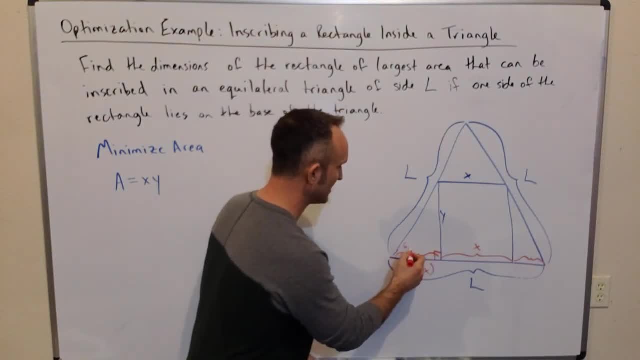 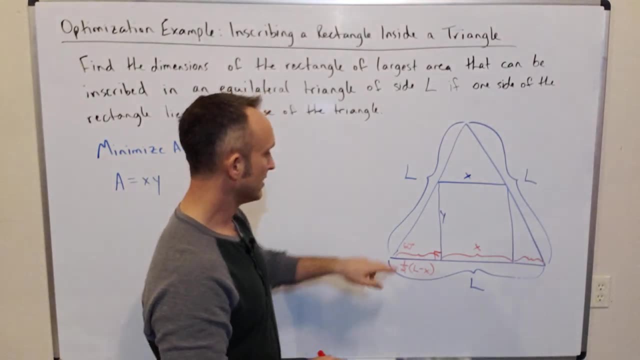 this is a 90-degree angle, but we also know that this is a 60-degree angle, because all three angles in an equilateral triangle are 60. They have to be equal, okay, So this is 60 degrees. And now we 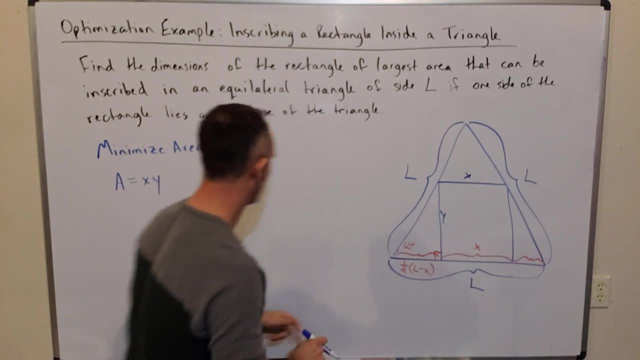 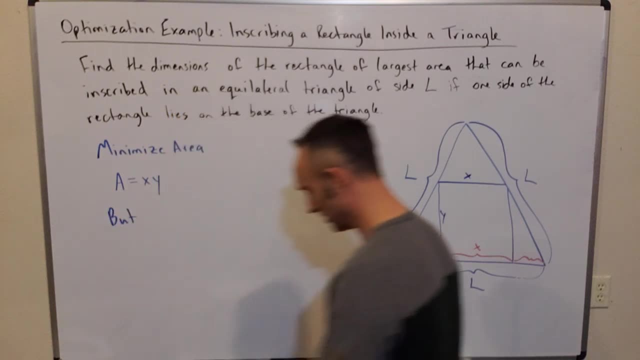 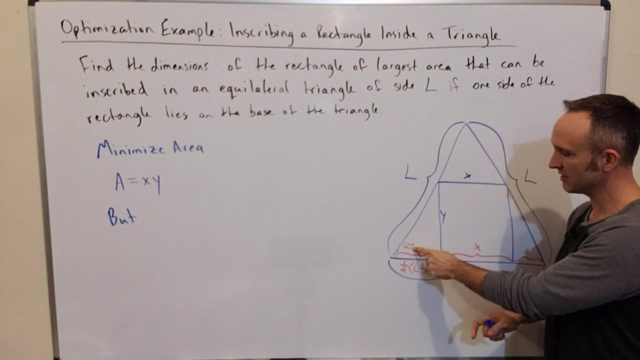 can get the relationship between X and Y, So let's write it over here. But if I'm using some trigonometric ratios and I'm dealing with this right triangle, with this acute angle of 60 degrees, I've got my opposite side and my adjacent side. I can set up a tangent. 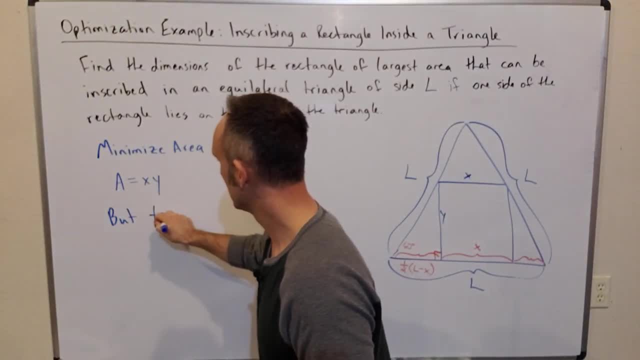 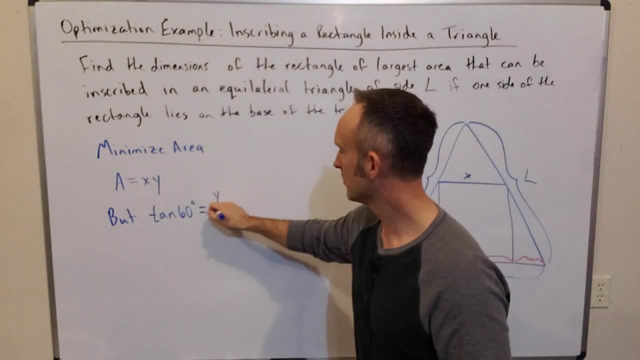 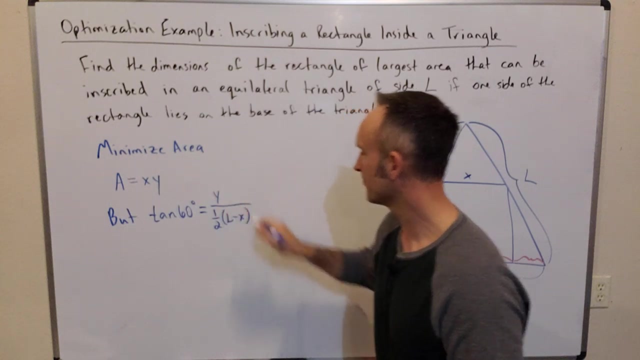 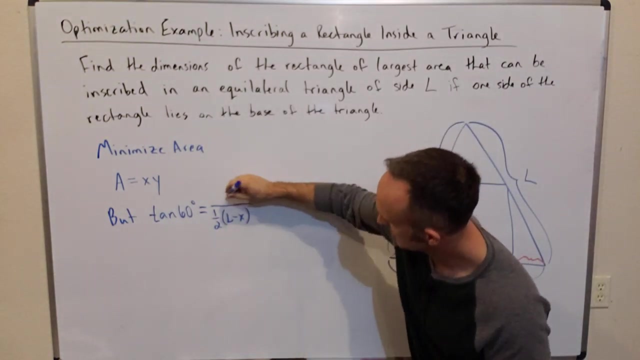 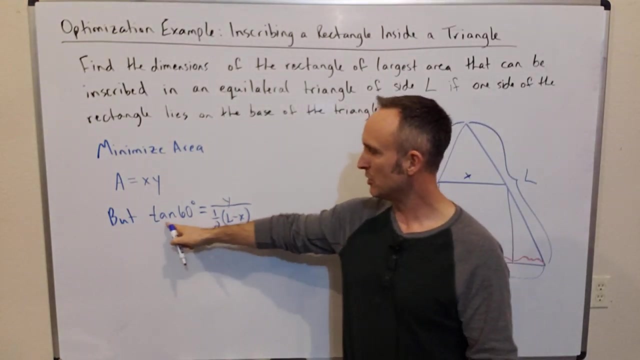 ratio and say that the tangent of 60 degrees equals the opposite side, Y, over the adjacent side to the quantity L minus X. And the cool thing about this is this makes it very easy to solve. Let me move my Y over here. This makes it very easy to solve this equation for Y. In fact, if you use 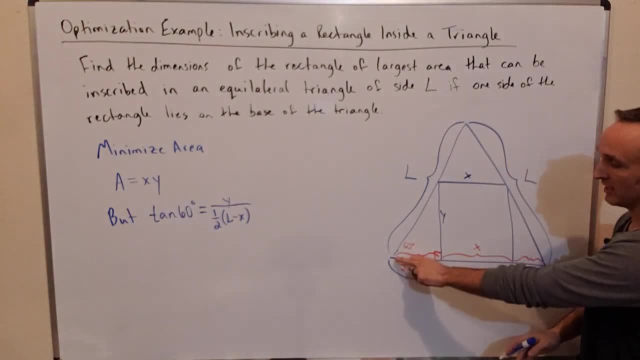 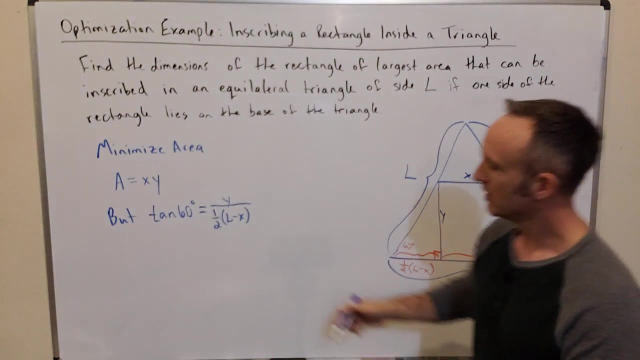 your calculator the tangent of 60 degrees. if you already recognize this is a 30-60-90 triangle, you probably know a little bit about those. If not, depend on the trigonometry here. But the tangent of 60 degrees is just. 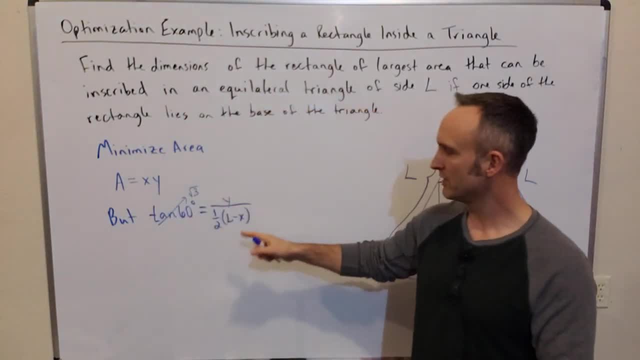 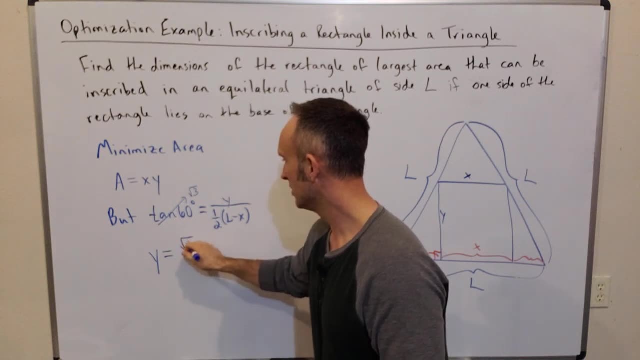 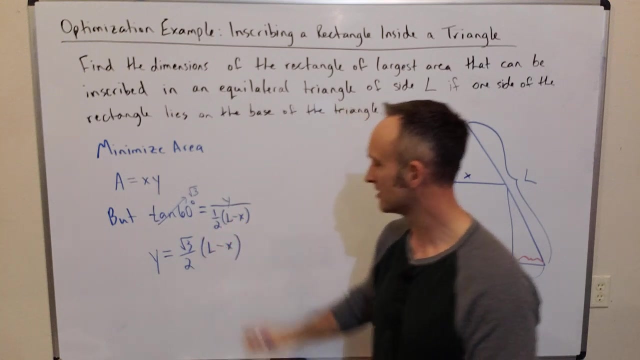 the square root of 3.. So if I solved this for Y, I would multiply both sides by my denominator. so I can see that Y equals the square root of 3 times 1. half is the square root of 3 over 2 times L minus X. 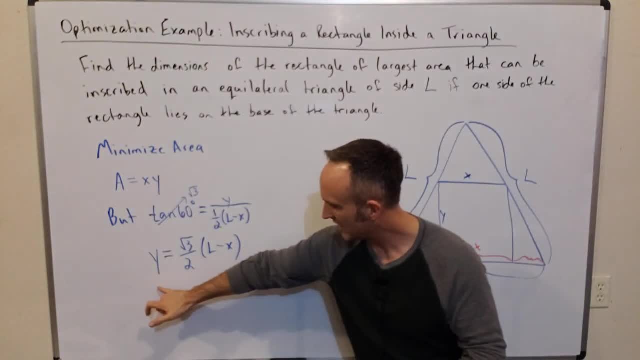 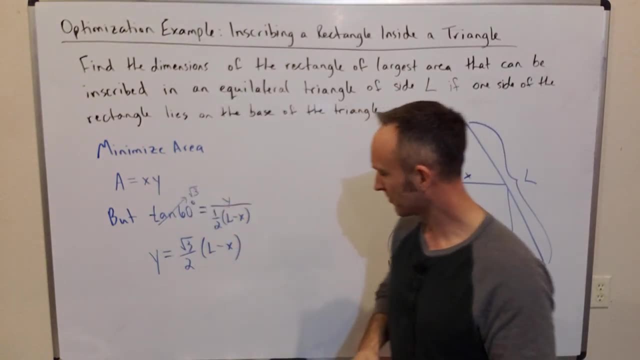 And remember, L is a constant, So we've taken Y and we've written it in terms of X And using that thought process, I can now come back and I can rewrite my area function. so I'm just going to tack on to the side. 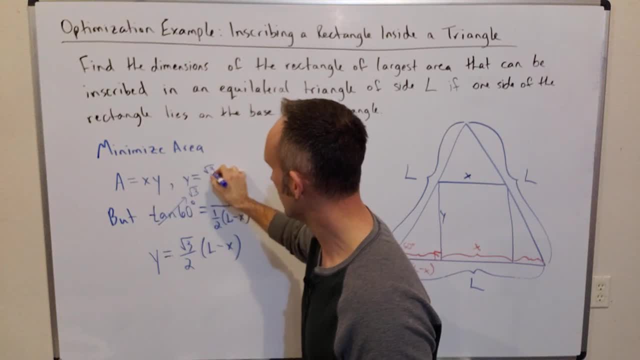 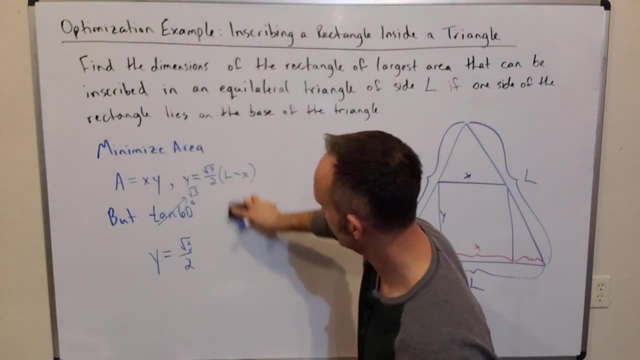 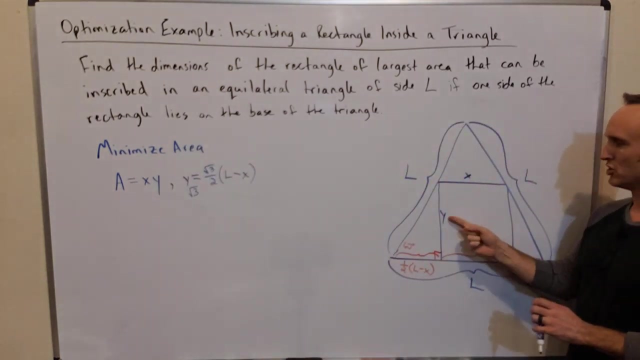 here in case we need it later- that Y is the square root of 3, over 2 times the quantity L minus X, and I'll erase our work for showing that. so I had to sort of I had to be creative in my diagram to find a relationship between Y and X and 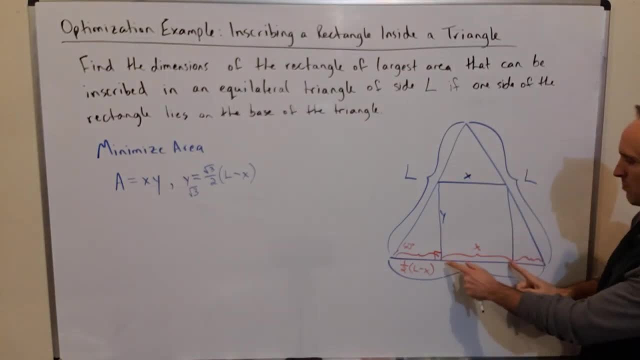 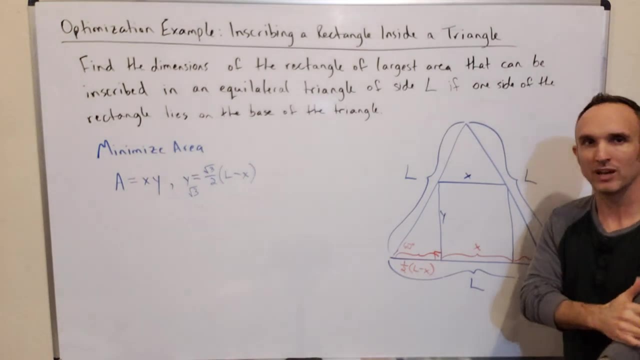 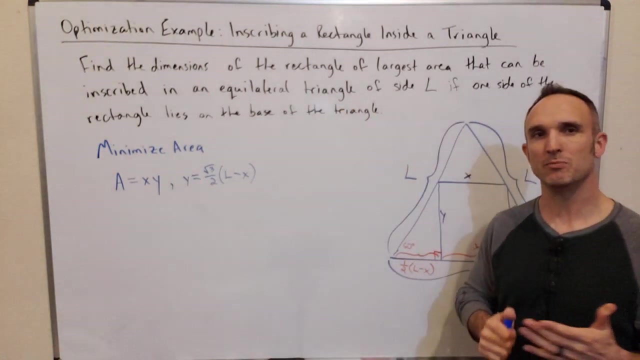 the way I did that was to translate X down to the bottom part of the rectangle, because then I could relate X and L, and that translated to my triangle, where I knew an angle. okay, so it's not at all obvious. so when you're solving these optimization problems, you really have to look for geometric, trigonometric. 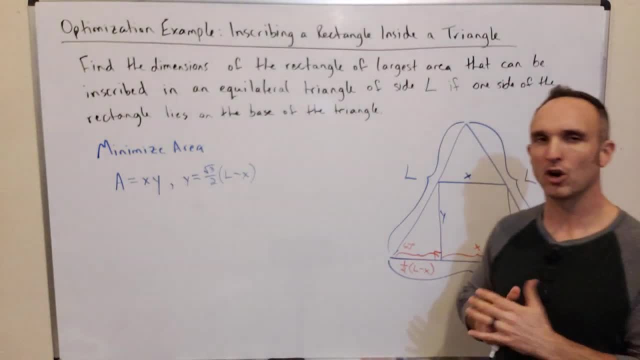 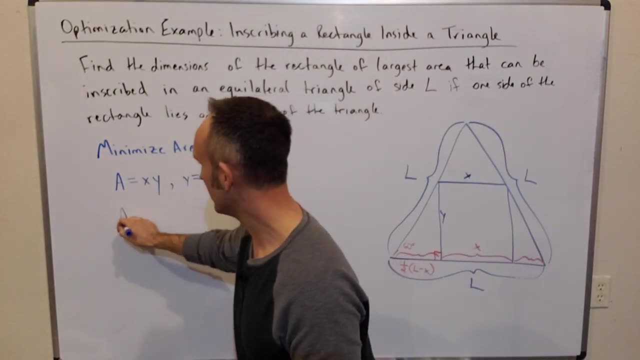 algebraic relationships and that that may be the hardest part of these types of problems. but now we've got. we've gotten past that. now I can rewrite my area function in terms of one variable, and that would be X, because this turns out to be a square root of 3 over 2 times the quantity L minus X, and that's 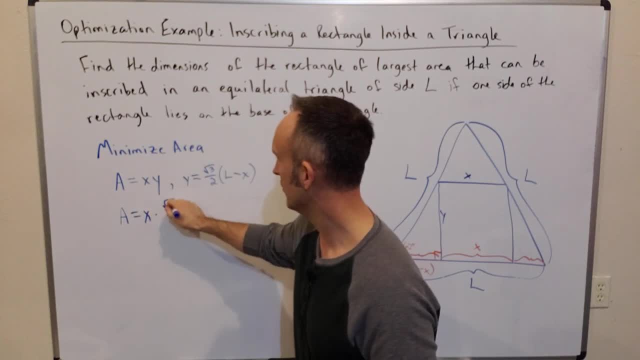 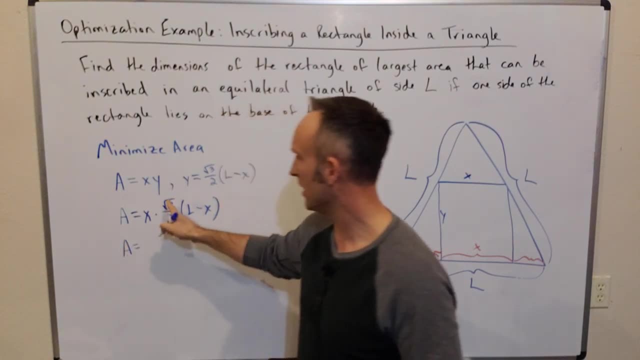 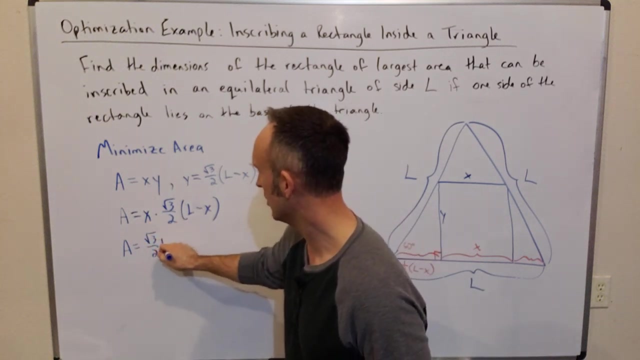 turns into X times Y, which is all of this. so if I distribute my X and my square root of 3 over 2, I get square root of 3 over 2, L times X. right, if I distribute these two guys to the L, I get this. the reason I'm putting it in this. 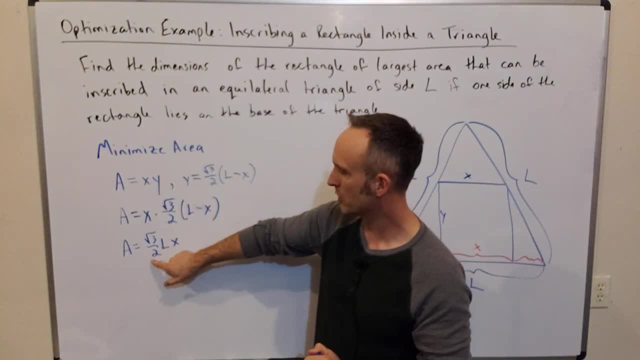 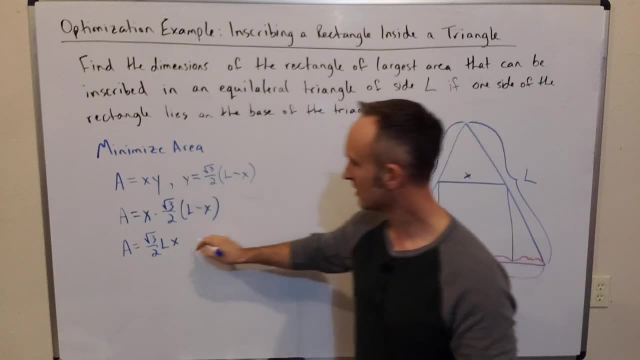 format is because X is my variable, whereas the square root of 3 over 2 and L are constants, so I'm absorbing my constants into the coefficient of my variable, X minus. if I distribute both of these to my negative X, I get square root of 3 over 2 as my 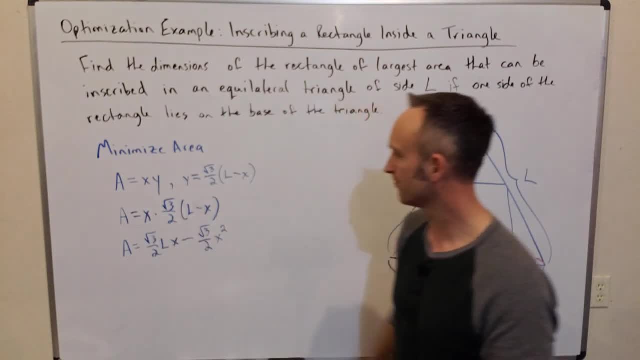 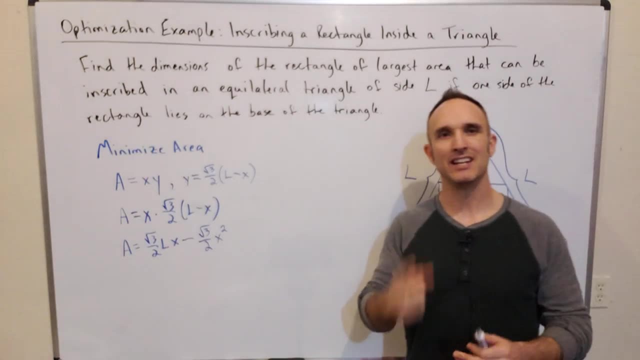 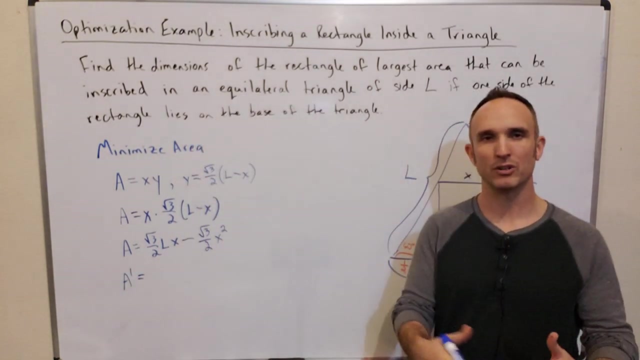 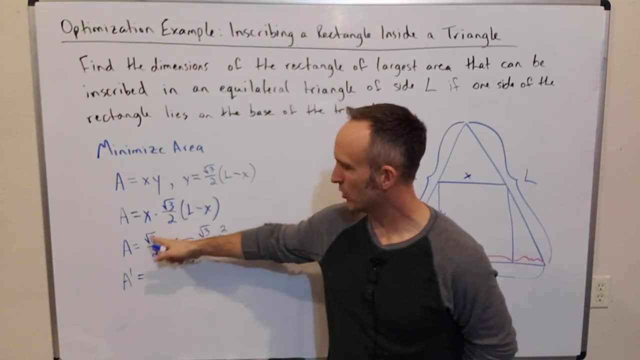 coefficient times X squared. okay, so now I have my area function as simple as it can get in terms of a single variable. so now I need to differentiate, find the critical numbers and hopefully max out my area function, maximize this area. So, differentiating this, I'm going to carry my coefficient and differentiate. 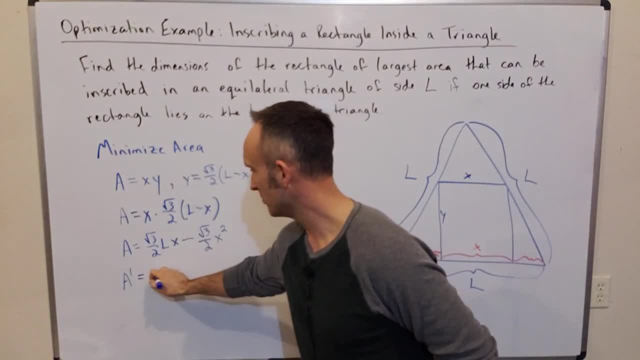 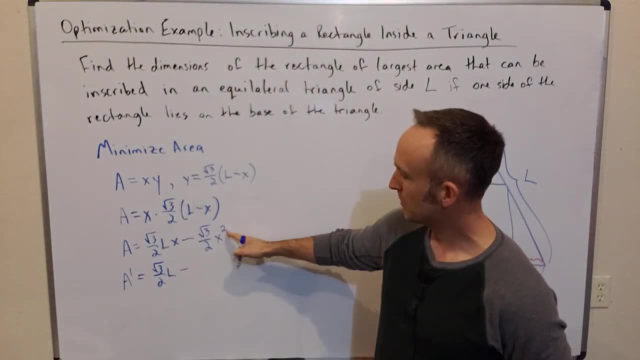 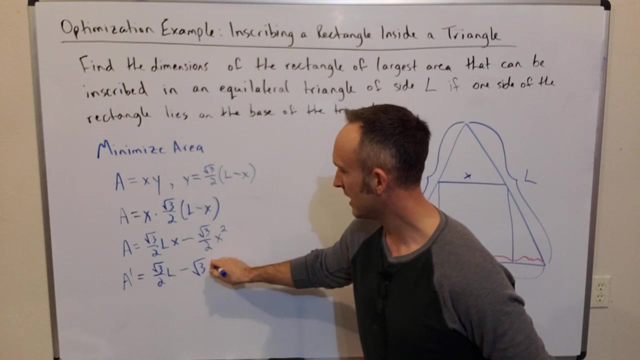 x just to get 1.. So the derivative here just simplifies down to the coefficient: square root of 3 over 2 times l minus power rule tells me to multiply my 2 by my coefficient. So I just get the square root of 3 and then times x to the subtract 1 from the power, so x to the first. 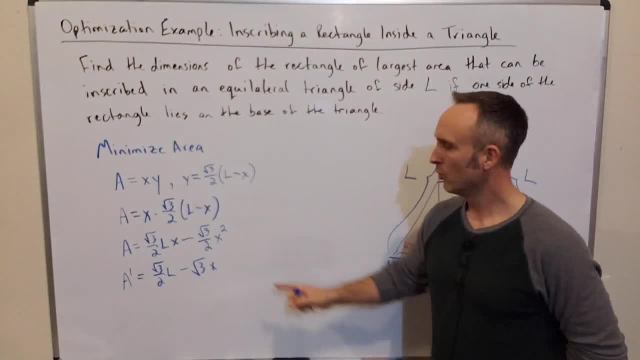 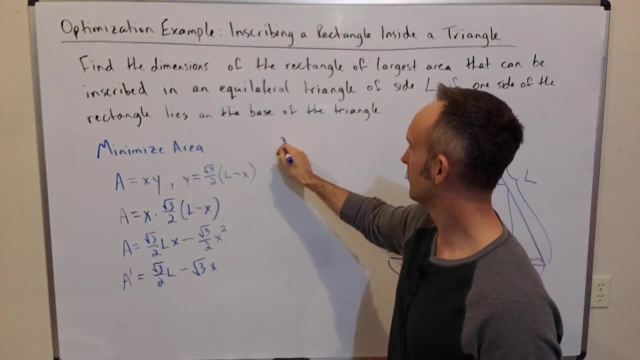 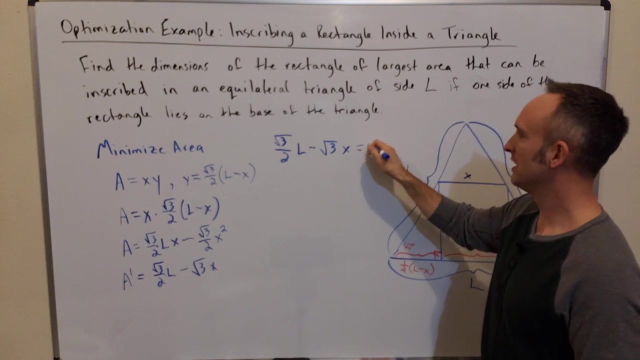 power, And now I have my derivative. Once I have my derivative, I need to find the critical numbers. So I'll set this equal to 0.. I'll set that equal to 0 and solve for x. right x is my. 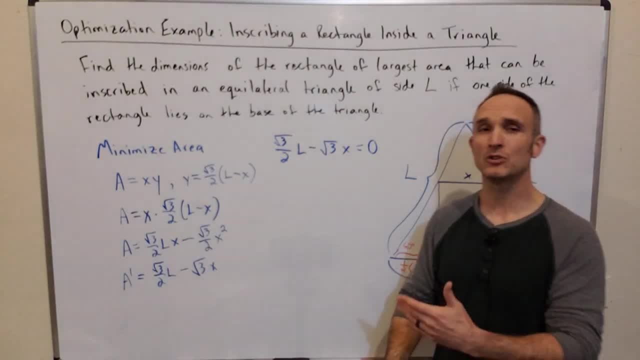 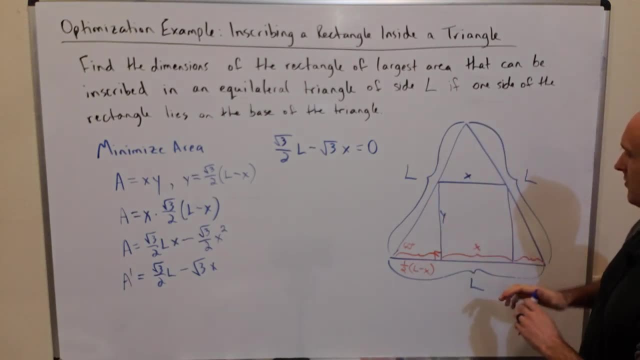 variable. here l is a constant. I know that's difficult to keep in mind. That's one of the reasons I chose to illustrate this example, In addition to the, the sort of curvy path you have to get to to get the equation in the first place. All right, 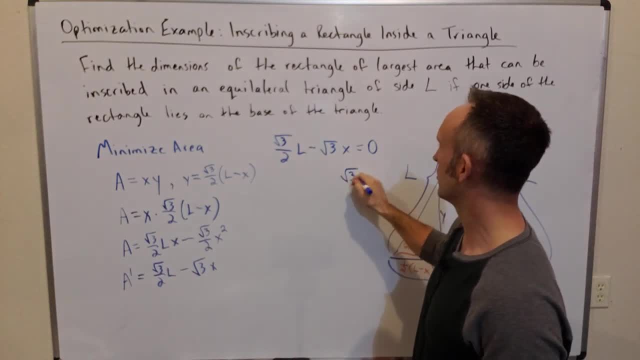 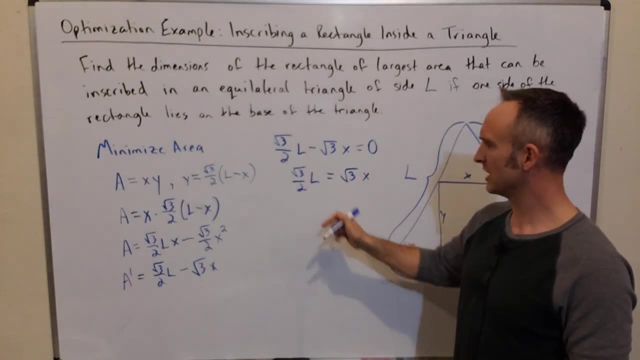 so if I solve this for x, let me add the square root of 3 times x to the right side and to the left side, And then I'll divide both sides by the square root of 3, which will just cancel this square root of 3.. So x is 1 half l or l over 2. I don't know which one's going to be better. 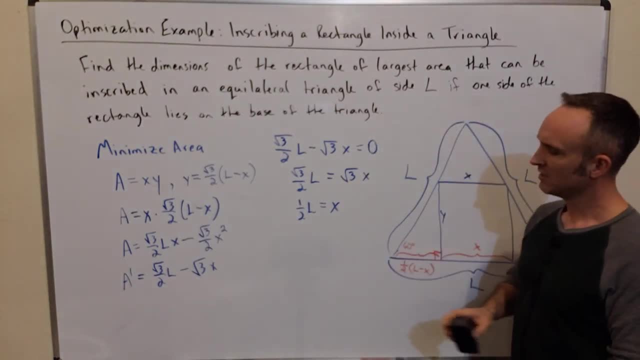 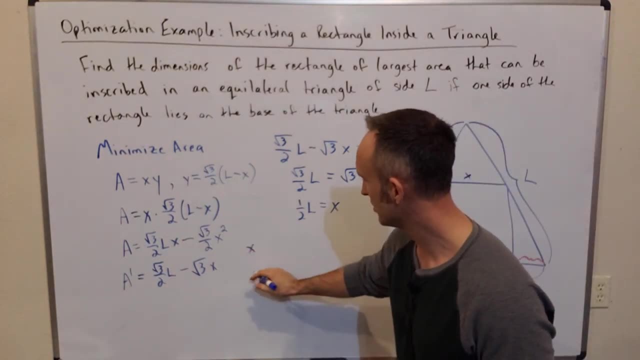 for us at this time, but I like 1 half l, So now we have to. we have to set up our chart. So I've got my x values, I've got my a prime, my derivative, and I've got my area function. 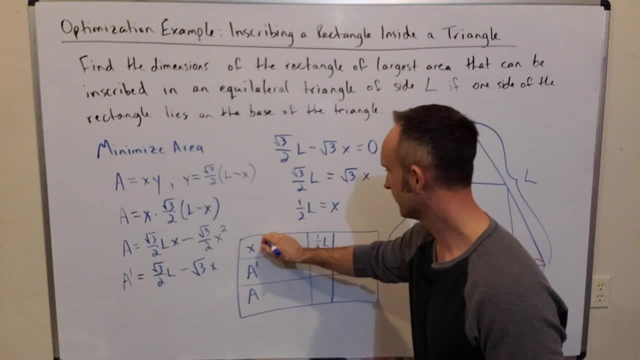 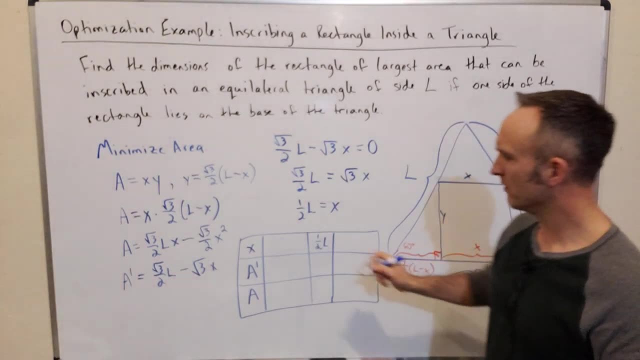 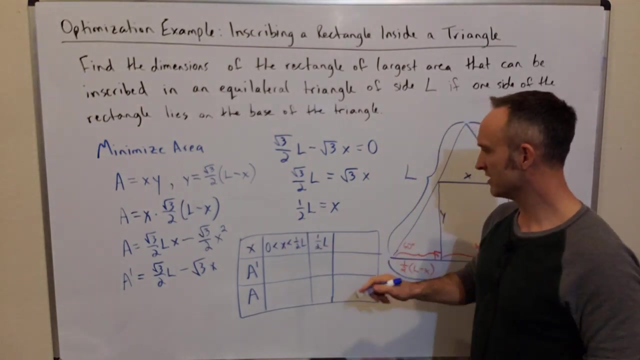 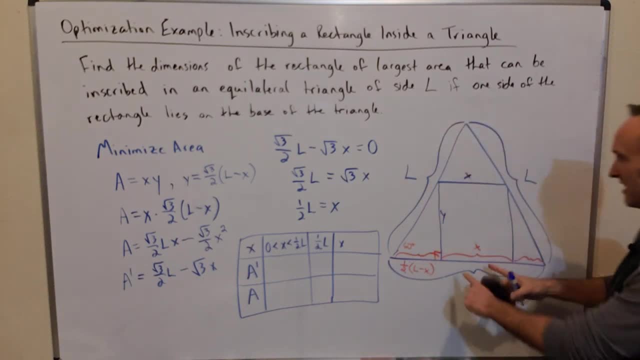 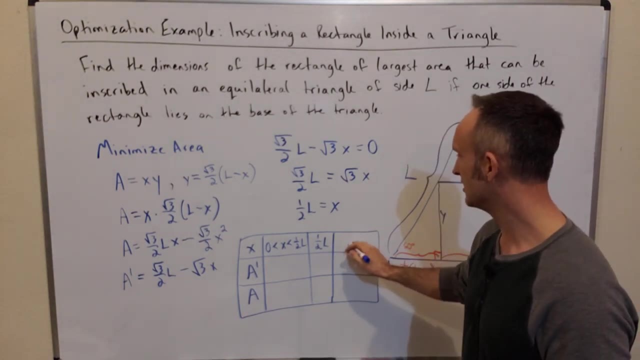 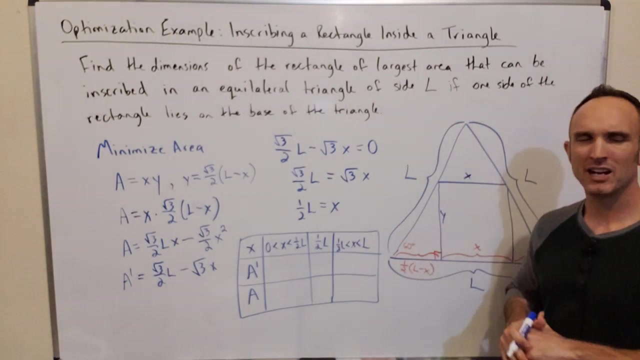 this side, X is in fact the biggest that X could get is L. it can't quite get there either. so on this side I will say: well, X is bigger than 1 half L, but it has to be less than L. okay, so you may try it. you may not catch that, but it's. 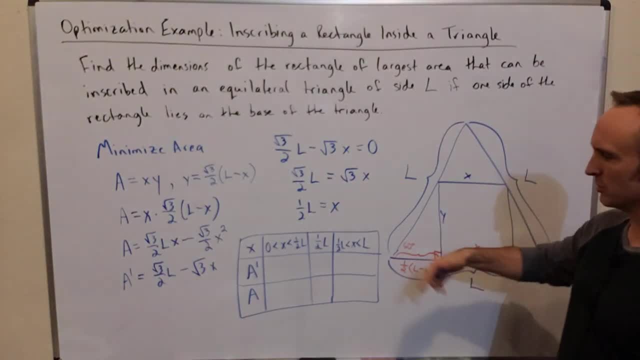 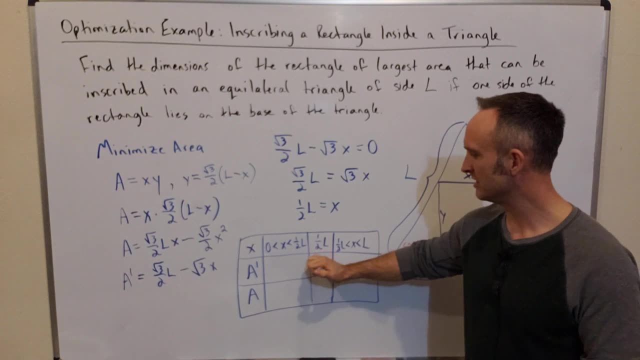 it's good for me to point out in these videos so that, so you're exposed to the right way of thinking as often as possible here. all right, we already know that a prime is 0. whenever X equals 1 half L, the derivative is 0, which means: 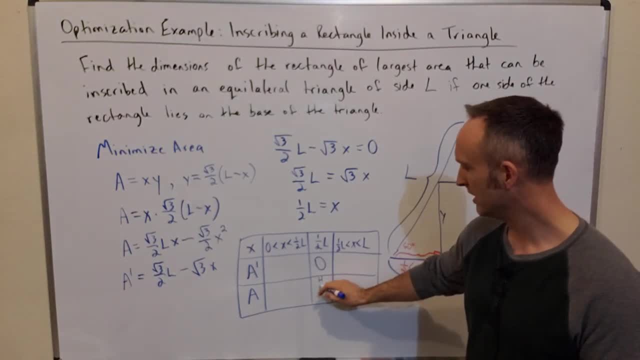 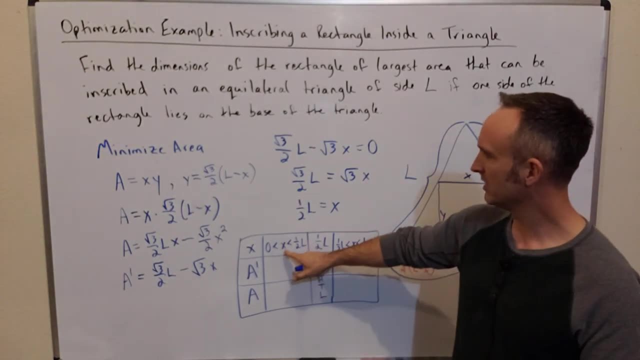 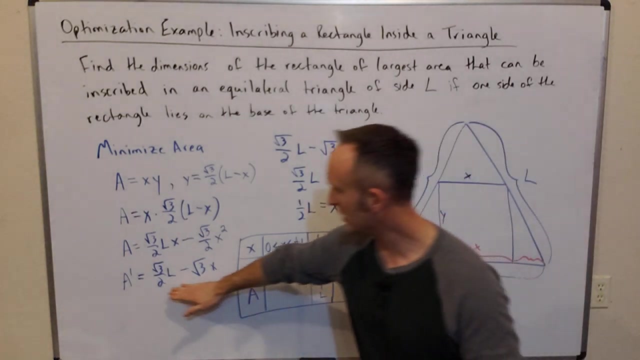 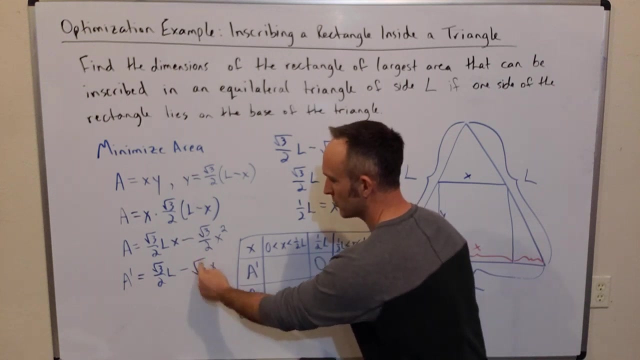 that the area of the rectangle would be would have a horizontal tangent line if we were to graph the curve for the area. function you, if I plug in numbers less than 1 half L into my- yeah, into my- a prime, then I'm going to get something smaller than the square root of 3 over 2 here. square root.